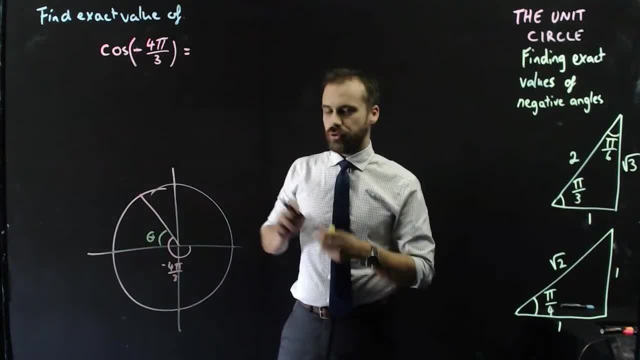 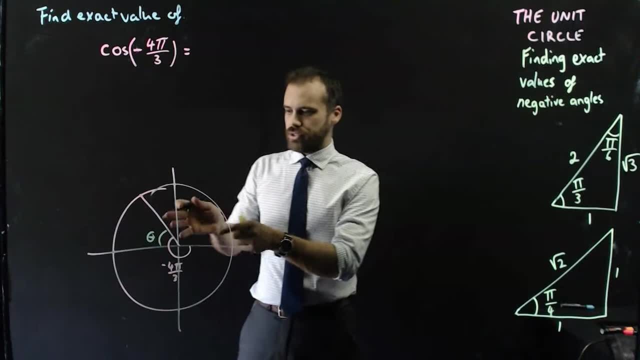 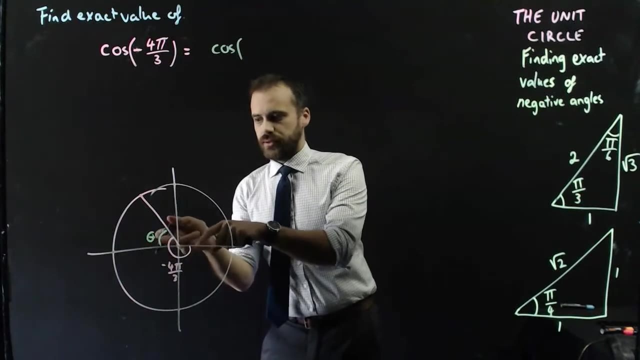 We're going to find that right there. Now, how can we find that? Well, it's up to you how you find that, But really probably the easiest way for us to do that is to understand that it's equal to pi minus this stuff. 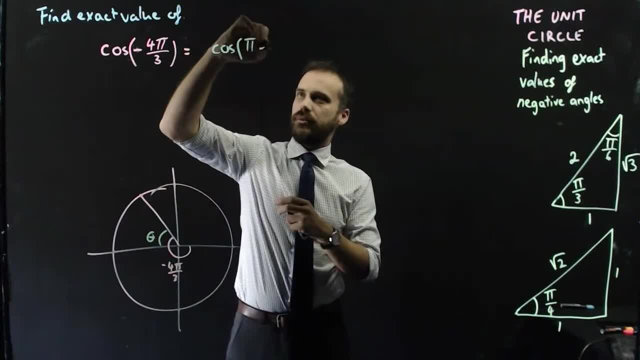 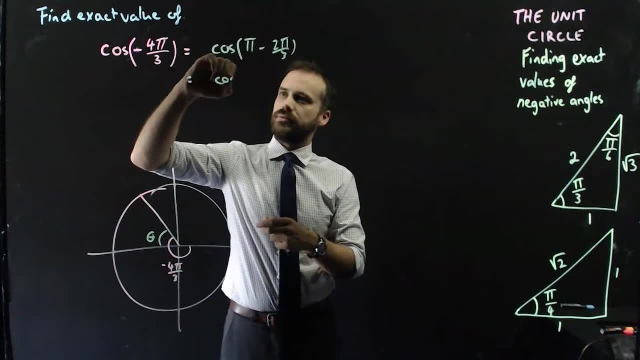 Or there's a few different ways you can do it, but let's do it that way: Pi minus 2, pi on 3. So that's equal to pi on 3. You can kind of skip that step and go to there, as long as you can clearly see what the angle is. 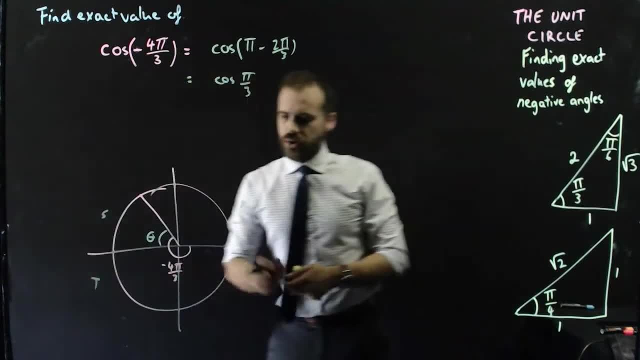 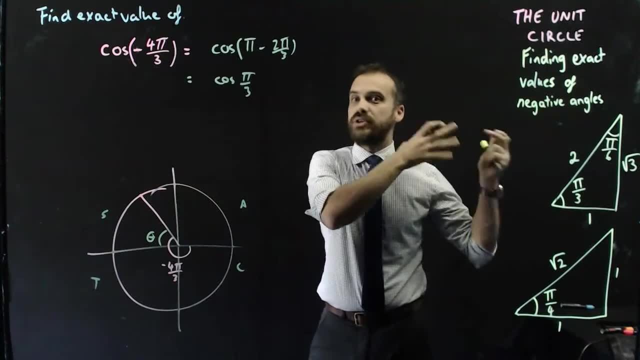 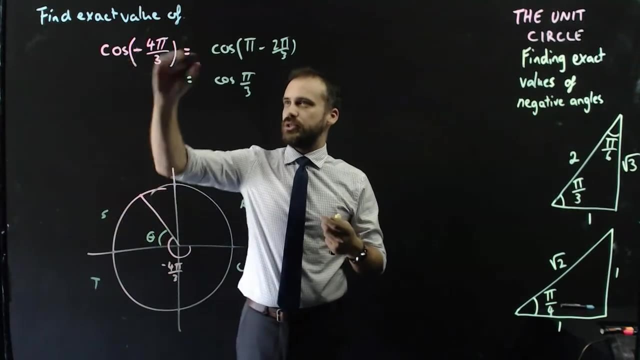 Now c a s t That negative has no bearing on this step. Once we've actually identified the angle, we're done with like the difference in this question with negative angles. So we can just say, well, we're in the s quadrant, but it's a cosine question, so it must be negative. 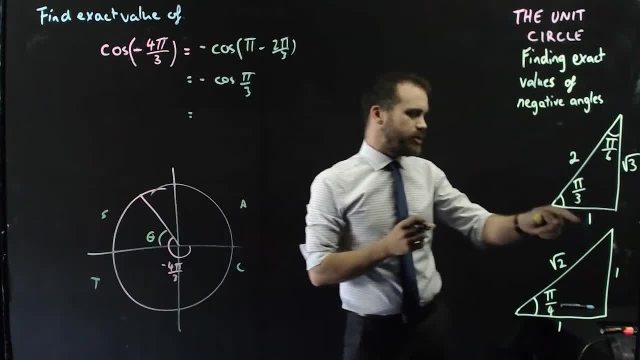 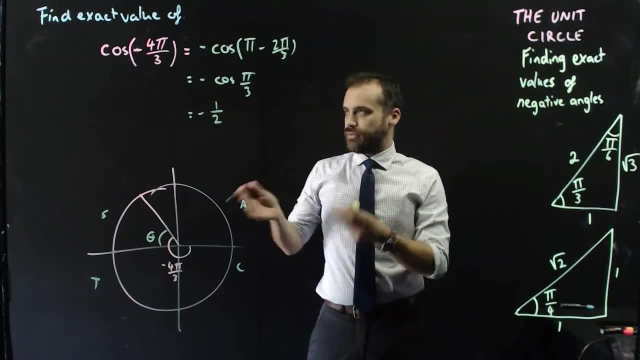 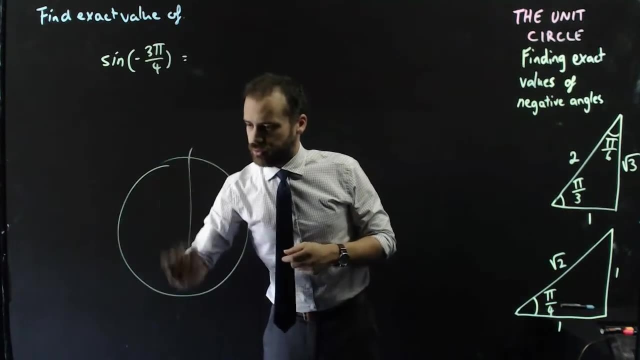 And then we go over here pi on 3, cosine, so adjacent over hypotenuse 1 half. But it's negative. So negative 1 half For that question, Alright. so again, it's just a negative angle. so unit circles, we're always drawing them. 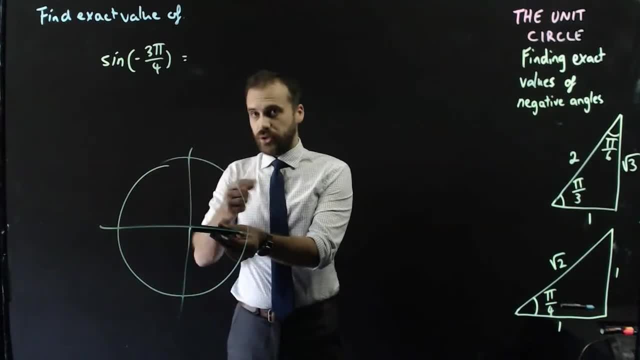 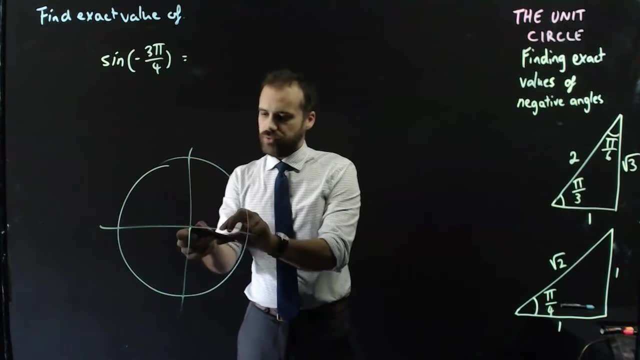 We start at the x axis and instead of moving anticlockwise like we have, we move clockwise because it's negative, So negative: 3 pi on 4, that's 1 pi on 4,, 2 pi on 4, 3 pi on 4.. 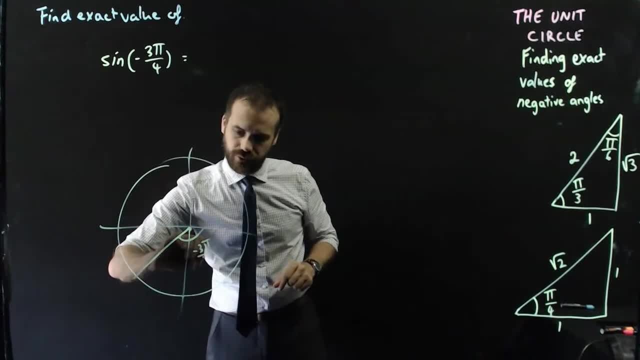 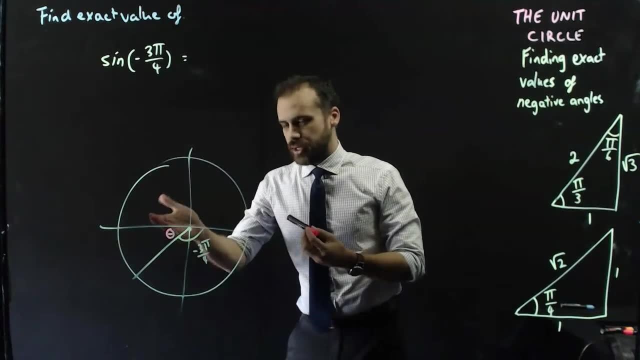 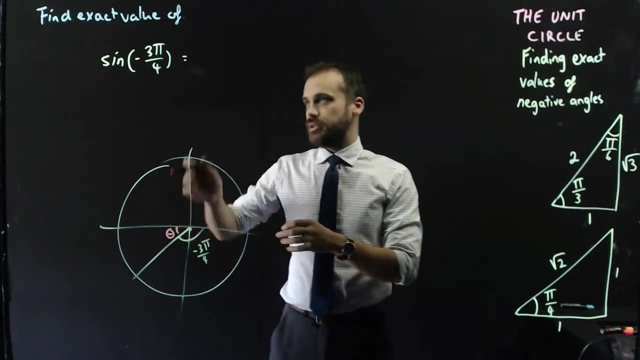 So that angle there represents negative 3 pi on 4.. Now we need to find our reference angle, which is, of course, this angle, the angle between our x axis and this point here. Okay, so now that we have our reference angle, we can say that that's equal to. I might just skip my next line here. 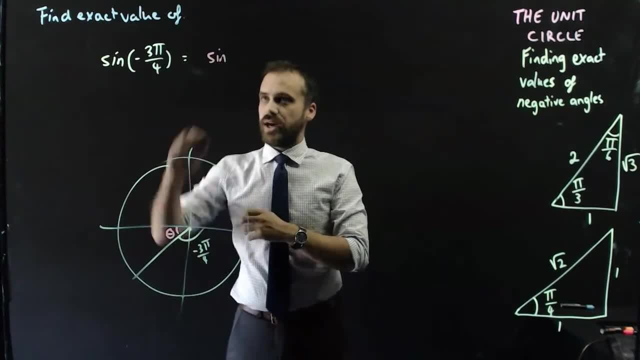 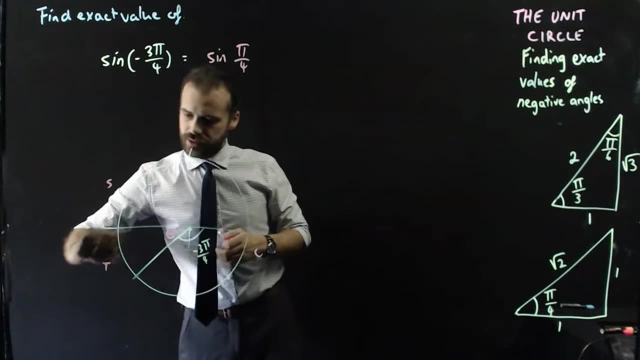 and just jump straight to saying that that is the same as whatever, that is, which is sine pi on 4.. Alright, now what quadrant are we in? C, a s T, so it's a sine ratio. in the T quadrant, so it's going to be negative.